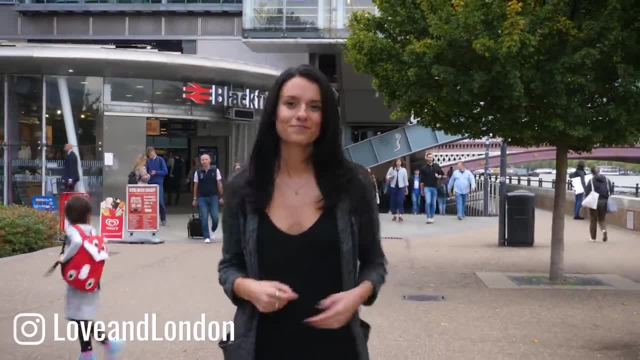 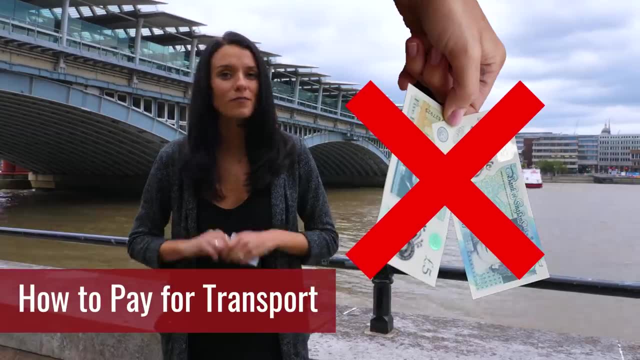 a special freebie for you at the end of the video, so keep watching. No, public transportation in London takes cash, so here are a few ways that you can pay for your rides. First up is an Oyster card. Get one of these, top it up, re-top it up when. 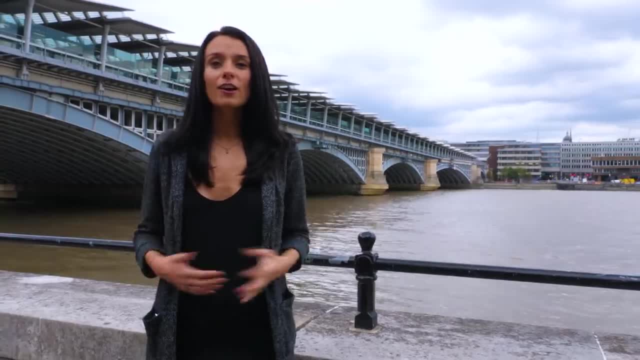 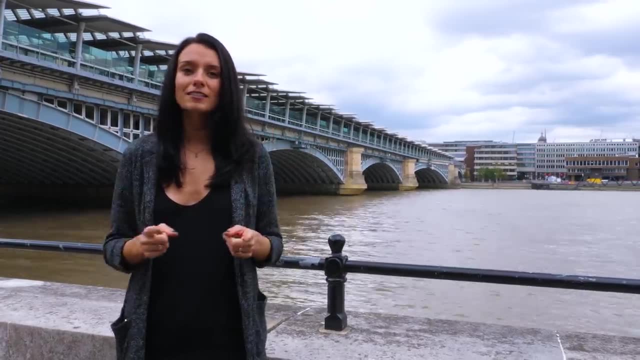 you need to, and that's it. You can also use your debit or credit card if it has the contact list feature enabled on it or if you have a card from outside the UK. sometimes the contact list feature and mobile pay doesn't work. 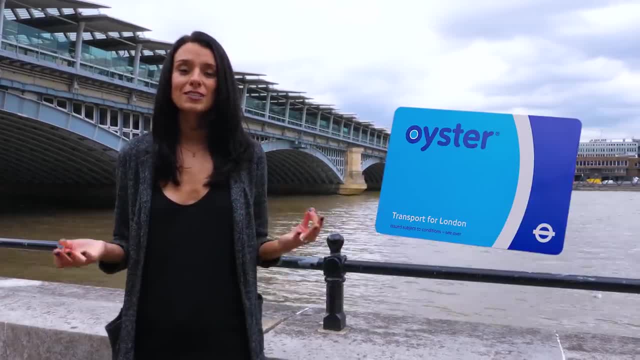 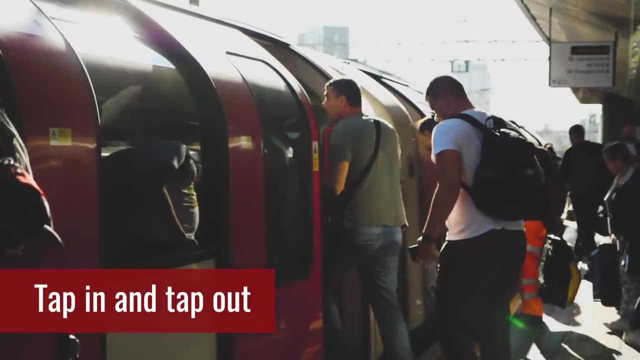 So I usually recommend for people to just get an Oyster card. It's the easiest way and the most reliable. You need to tap in and tap out. When you're taking a train or the Underground in London, you always have to make sure you tap in at the first station you get on at and tap out. 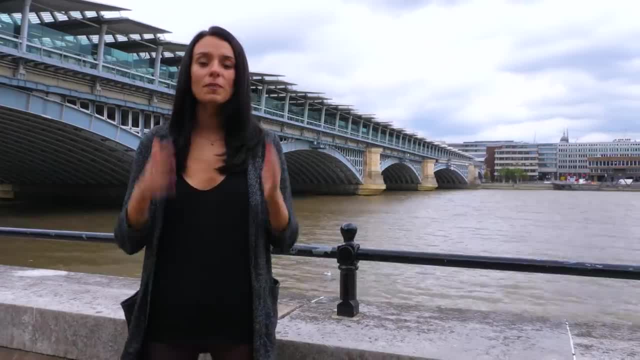 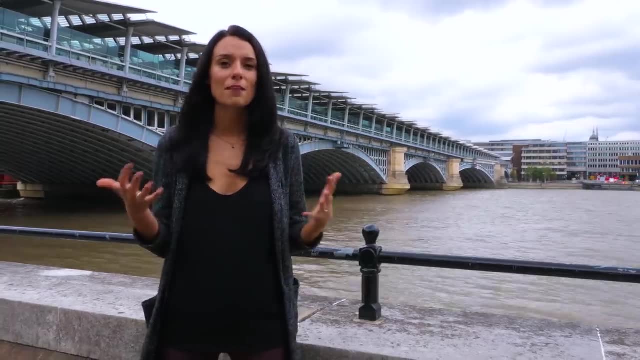 at the station that you leave at. This is because you get charged depending on how much distance that you travel. Most of the time you're going to hit barriers to get into the station and out, so you'll know that you need to tap in and tap out, but sometimes at night. 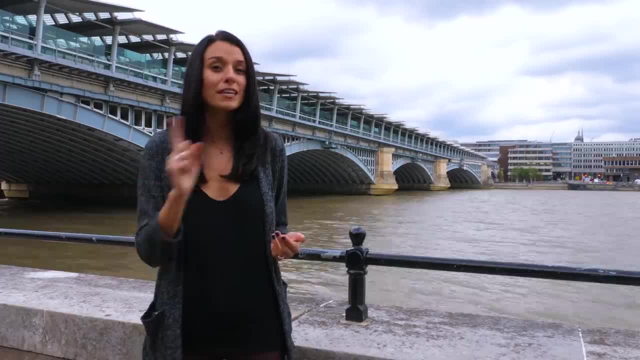 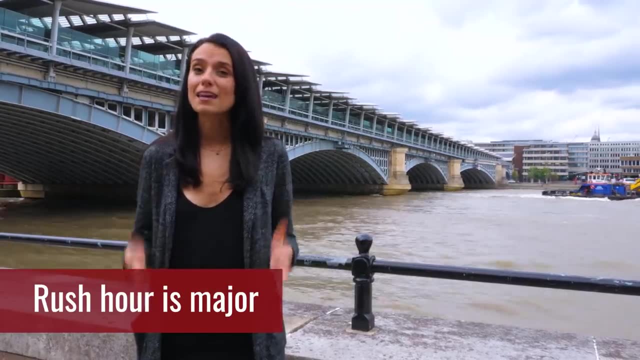 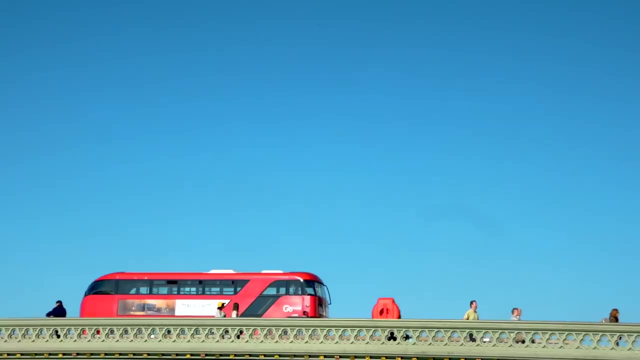 they leave the barriers open. So make sure you still tap in and tap out even if that happens. Rush hour is major in London, so try not to travel on public transport at those times if you can. You will avoid major crowds and major traffic. Try to walk if you can. 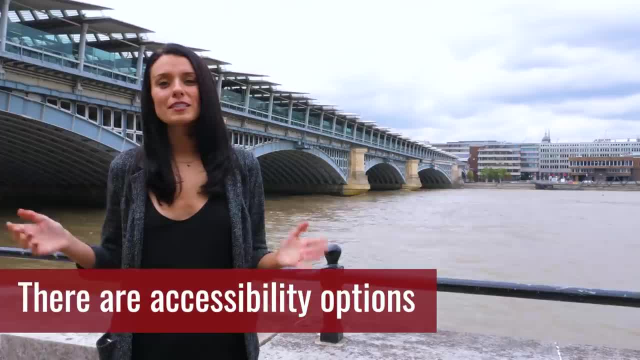 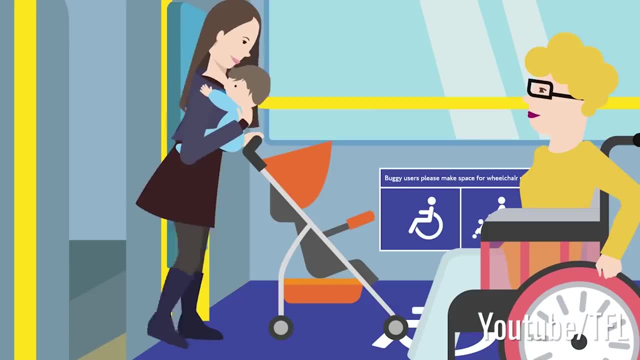 If you need to avoid steps when getting around London, the buses are always going to be your best bet, because they're equipped with ramps and wheelchair accessible seating. You'll also see on every tube map that the accessible seating is not available. You'll also see: 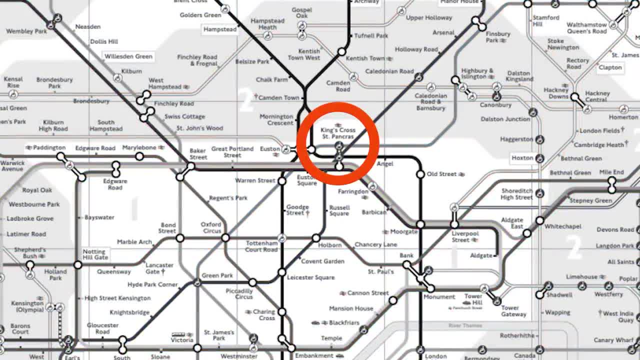 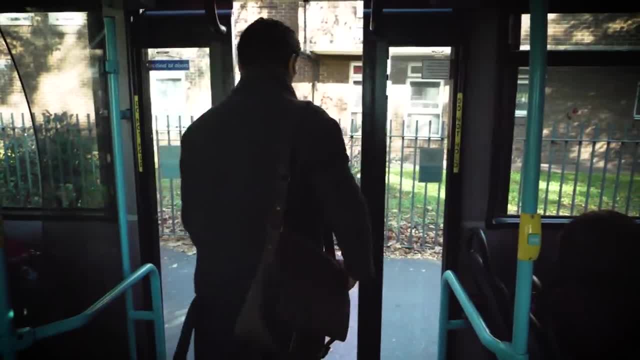 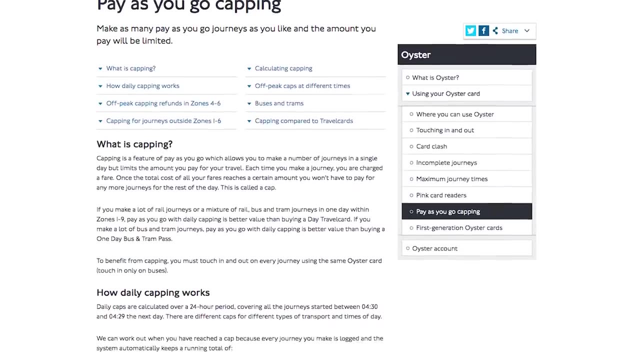 on every tube map that the accessible stations are marked off. If you have other accessibility needs, I've left some links down in the description of this video to other resources that will help you out. London's transportation system has a daily cap, which means if you travel a lot around, 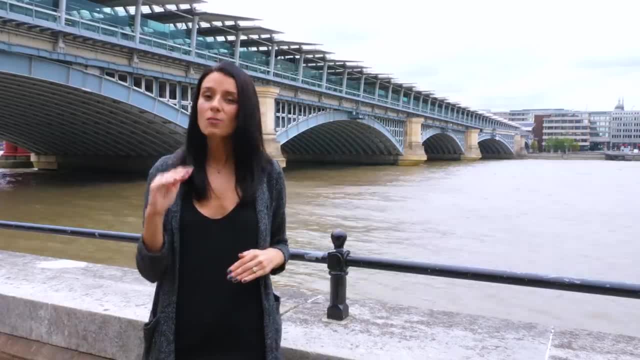 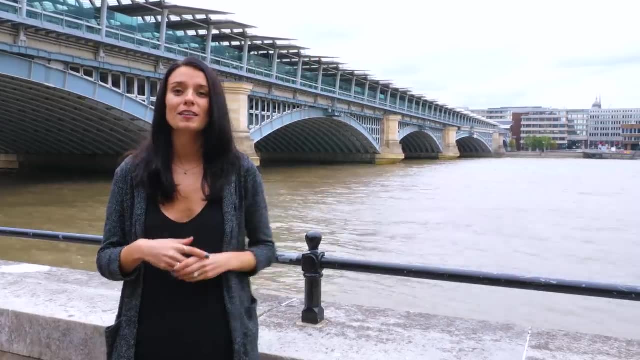 each day, you will only be charged a certain amount. How much you get charged depends on how many zones that you've traveled through, And if you don't know what zones are, you should watch the video that's popping up here in the corner. That will tell you all about. 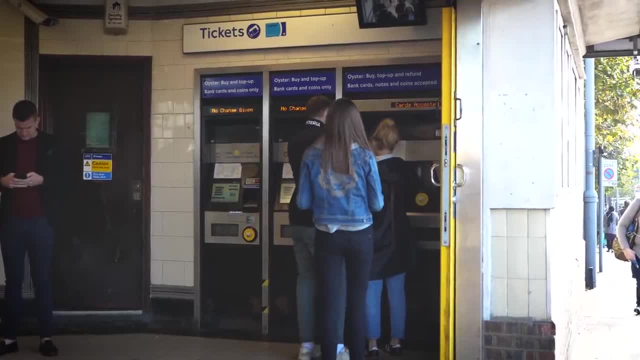 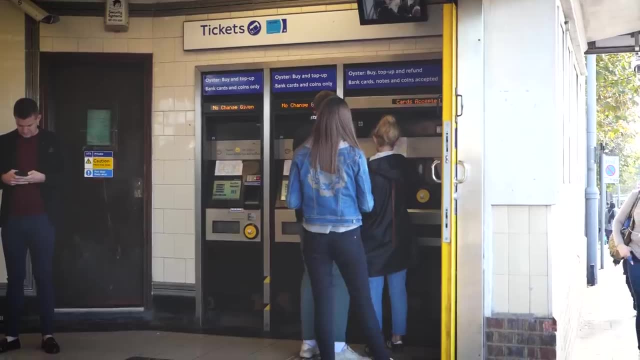 how zones work. If you're using an Oyster card and you need to check how much balance you have, there are two ways to do it. The first is to use one of the ticket machines in a station or when you tap out at a barrier. you'll see the amount of credit that's left on your card.